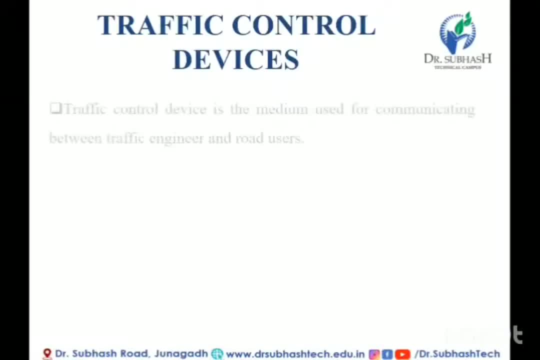 7agedb package. just call number three and click here, and then we let's start with the topic tomorrow. So in this video we are going to talk about properly knowing the capacity for 보: Vlog Signers, so traffic control device, So the. 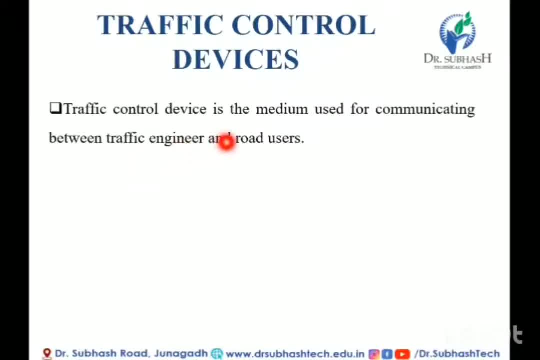 on the 4th giving of UK road user. the thing is we know that in order to get traffic. 5. The system of no traffic between public and non public students that happens in your region. opened in the imagery format: The mechanism or plausibility of No traffic sí. 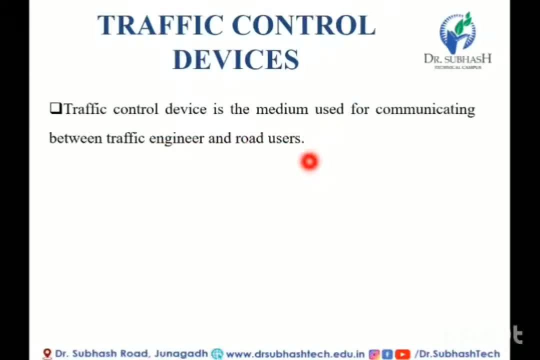 without causing any delay or any accidents. so so traffic control device is a medium which is used for communicating between the traffic engineers and the road users. now, this road traffic control device includes markers, signs and signal devices used to inform, guide and control the traffic, which also includes pedestrians, motor vehicle drivers and bicyclists. so traffic control device. 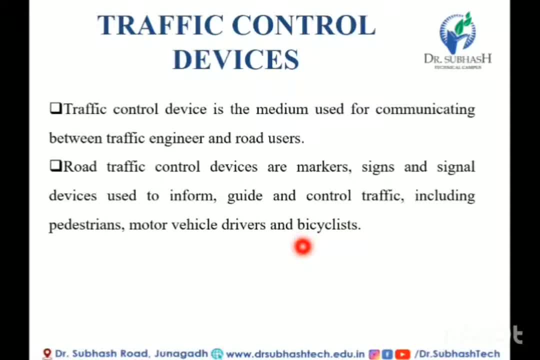 includes several facilities or several things, like traffic signs, traffic signals, then road markers. now this particular device is used to inform, guide and control the traffic, which includes the pedestrians, bicyclists, as well as motorcycle or motor vehicle drivers. now these devices are used are usually placed adjacent over or along the highway road. 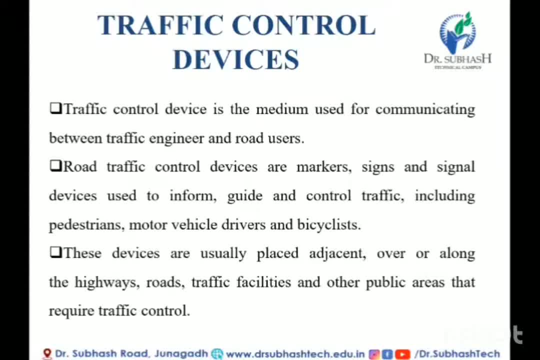 traffic facilities and other public areas that require traffic control. so traffic control device are placed on that particular road where traffic control is required. so the traffic engineer will carry out several surveys, traffic related surveys, in order to address it the need of traffic control device in that particular road, after identifying 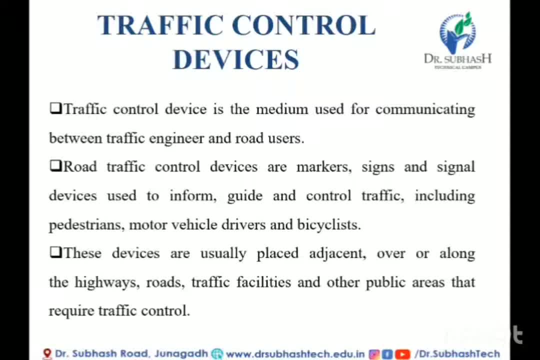 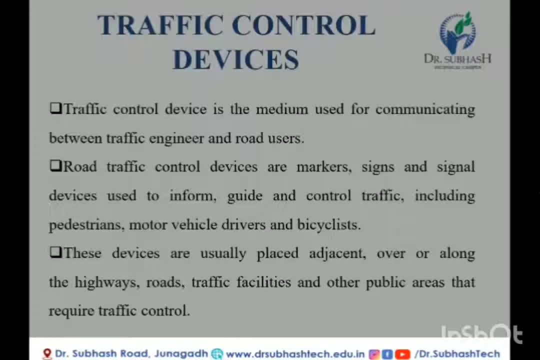 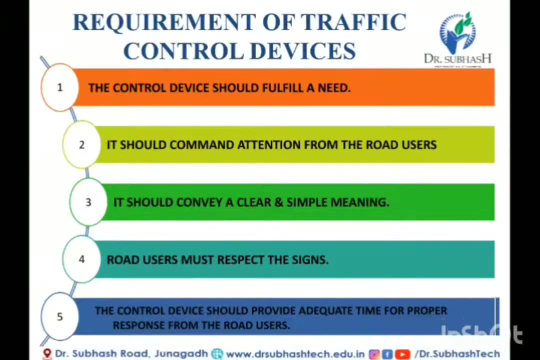 the need, the various types of traffic control devices are installed. now let us see the requirement of traffic control device. now the requirement of traffic control devices are. so there are five main requirements, or we can say five main objective or functions of traffic control device. so the first function is: 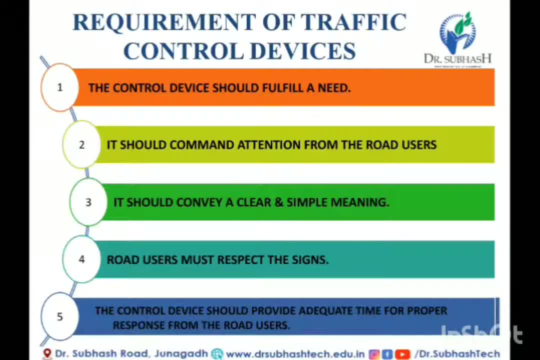 first one is the traffic control device should fulfill a need now. each traffic control device must have a specific purpose for the safe and efficient operation of the traffic flow. for example, if we are installing a traffic signal at the intersection, then it must reduce the continue to know that it will be resulting traffic control device in the traffic state. whereas in traffic state we reduce traffic control. local clock, clock signal, continuous autumn. these traffic signals will determine function of traffic flow. district Séptimes we can substitute traffic control Metro sized traffic ranges, environment different time. it is just a matter of few minutes. this is a situation. 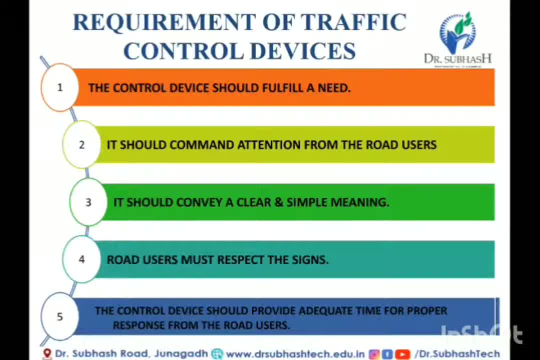 cost in that particular intersection, or else the road marking. if we are using any road marking, then that particular thing should give proper informations to the road users. now the second requirement is it should command attention from the road users. now this traffic control design affects the design of a signs for commanding attention. proper visibility should be. 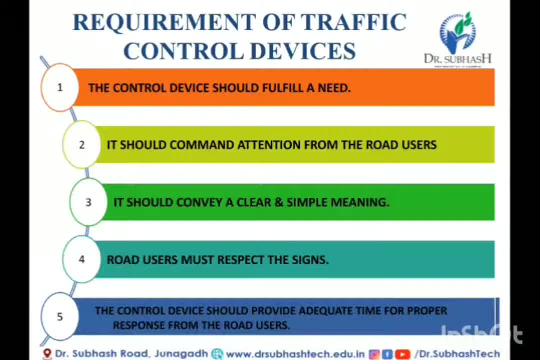 there so that the road users can properly see those traffic control devices. then only they can follow them properly. also, the sign should be distinctive and clear. the sign should be placed in such a way that the driver requires no extra effort to see the sign. now, in certain conditions, the road users may complain. 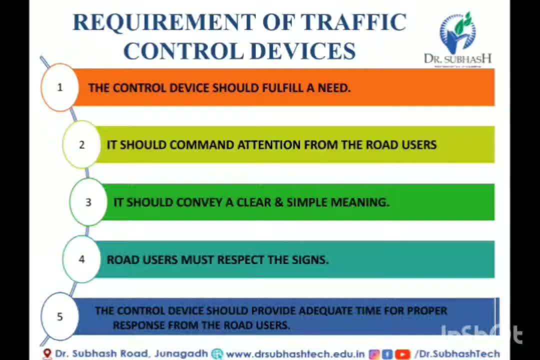 that he was unable to see the road traffic control device. so the traffic engineer should plan in such a way that the traffic control devices are installed in proper place, where it is clearly visible to the road users. now the third requirement is it should convey a clear and simple meaning or simple message. now 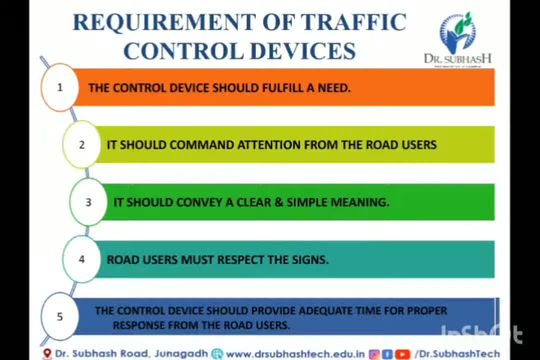 clarity and simplicity of message is essential for the driver to properly understand the meaning in short time, because the driver is also focusing on his driving and he has less time to see the traffic control device and read it. so the use of color, shape and legend as codes becomes important in this regard. the legend should be kept. 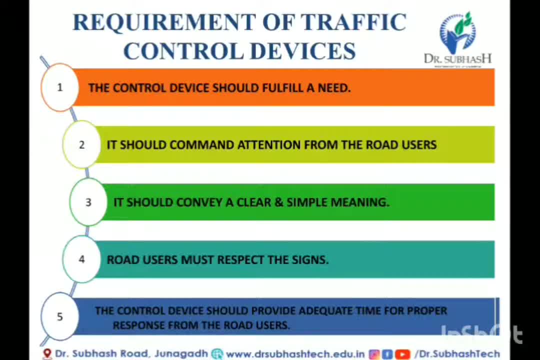 short and simple so that even a less educated driver could understand the message in less time. so that was requirement number three. now the fourth requirement is the road users must respect the science. now, respect is commanded only when the drivers are conditioned to expect or that all devices carry meaningful and important messages. the road users will only 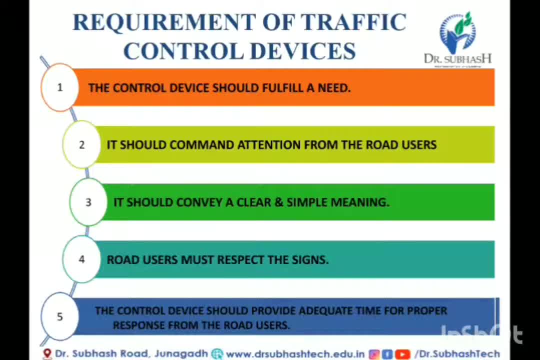 respect a traffic control device if it is fulfilled- fulfilling the need of the road users- or it may be soft, solving the problems of the road users, if it is reducing the congestion, if it is reducing the accident, if it is helpful for providing smooth flow of journey, then all the road users will respect the 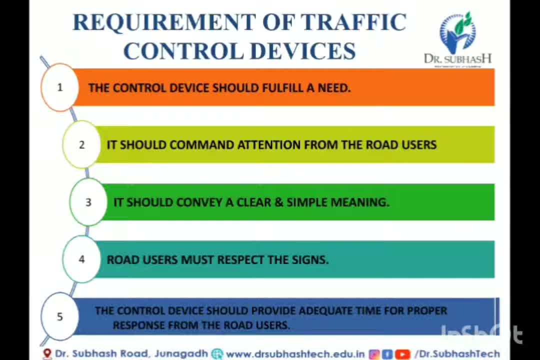 traffic control devices. and also we must remember that overview, misuse and cuisine messages of traffic control devices tends the drivers to ignore them. so that must be taken care properly, that the traffic sign should be clearly understood by all the road users. now the fifth requirement is the traffic control. 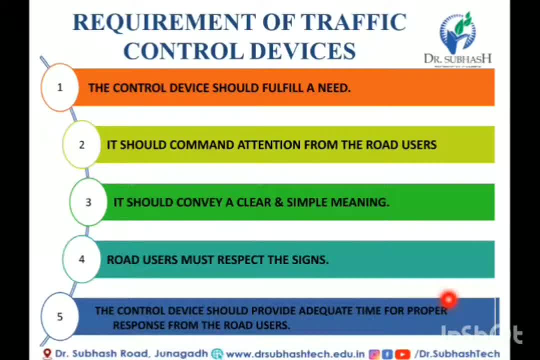 device should provide adequate time for proper response from the road users. now this is again related to the design aspect of traffic control devices. the signboard should be placed at a distance such that the driver could see it and get sufficient time to respond to the situation, for example, the stop sign. 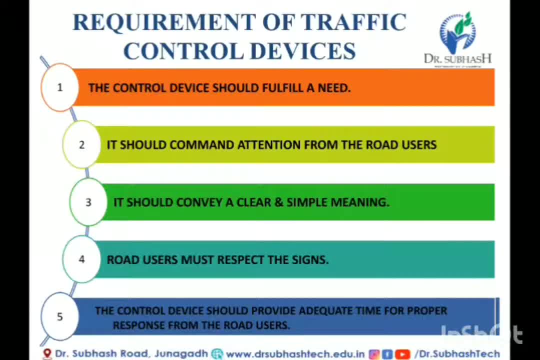 which is always placed at the stop line of the intersection, should be visible for at least one safe stopping sight distance away from the stop line. so we must also consider the braking distance. if we are using a stop sign just near the stop line, then they will not be able to stop the vehicle exactly behind the stop line. 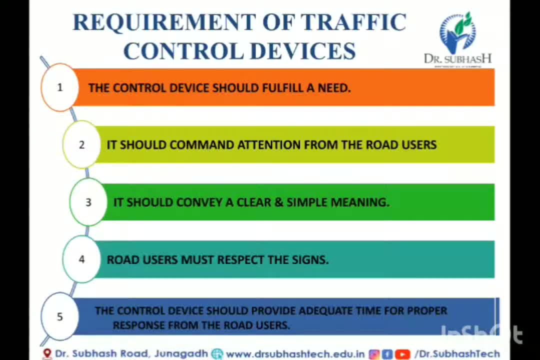 so distance is also important and the location of the traffic signboard is very important. so this were the five main requirements of traffic control devices. first one was to control. the traffic control device should fulfill a particular need. second, it should command attention from the road users. third is it should 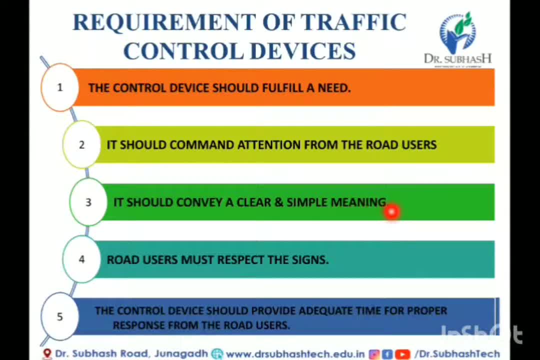 convey a clear and simple meaning or simple message. fourth one: the road users must respect the signs. and the fifth one: the control device should provide adequate time for proper response from the road users. so this were the requirement of traffic control devices. now moving to the next slide. 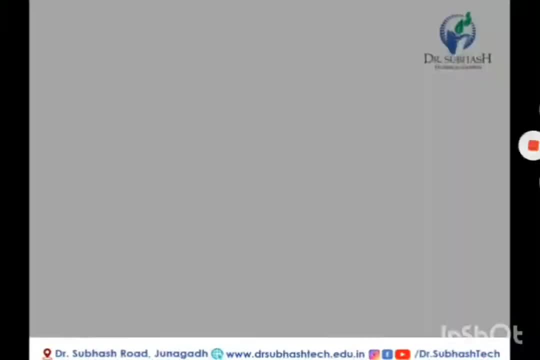 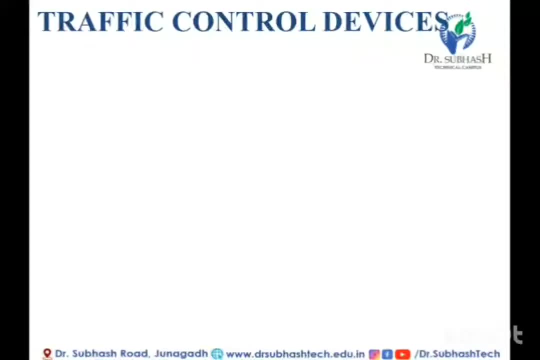 people's license to check your traffic connected to your station. let's look at some of the devices which are included, which are termed as traffic control devices. so there are four main devices, the various 8th and devices used to control, regulate and guide the traffic. of first one, science, traffic. 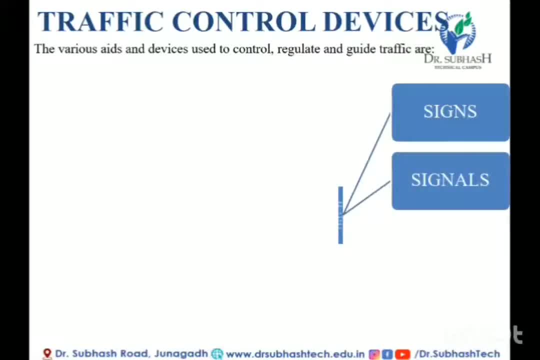 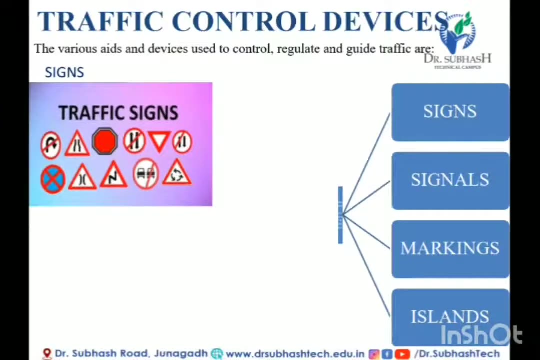 science. then second one is signal- stop signals, then road markings, and the fourth one is high lines. so, starting with signs, now understanding traffic. each and every type of traffic sign is among the most important aspect for all the road users. the traffic signs communicate the basic rules and regulations of the road through simple graphics. 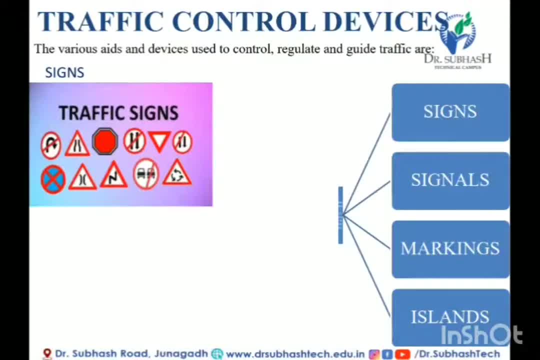 that can be understood within seconds. also, anyone who wish to apply for a driving license. they first need to learn all the traffic sign in order to pass the theoretical examination of driving. after passing the theoretical examination, then only you will be allowed to participate in the practical test of the vehicle. so 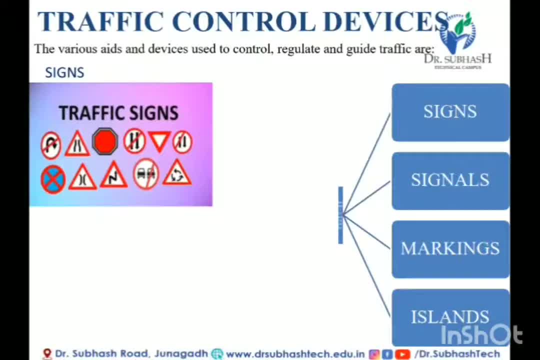 it is important for all the drivers to know about the traffic sign, or the road safety signs, in order to ensure the safety of himself as well as others. now, the basic functions of traffic sign include: it inform the road users of the distance left to cover to reach a destination. 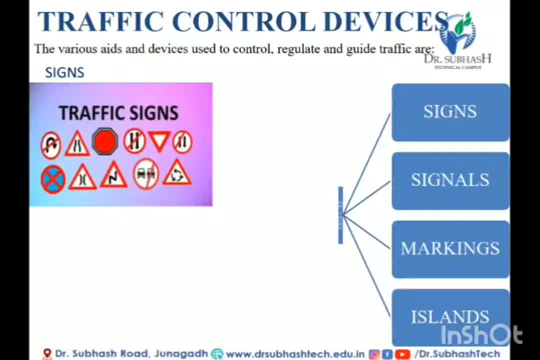 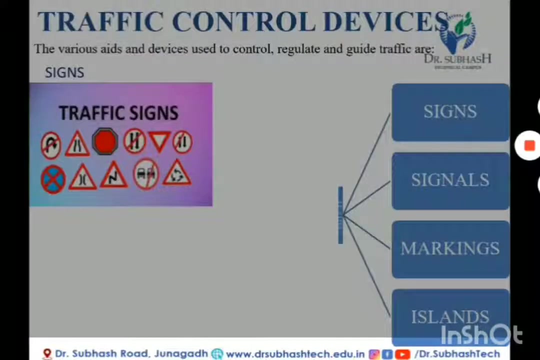 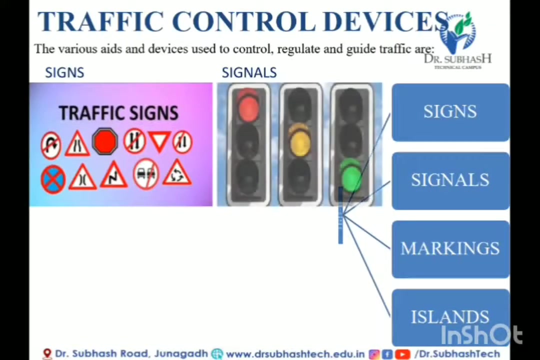 it also inform the road users of the alternative routes to a destination and the caution road users of hazard near areas such as schools and colleges. and it also inform the road users of specific locations, such as those of public convenience outlets, restaurants and hospitals. now the next device is signals. now traffic signals are given out by device that are mostly placed. 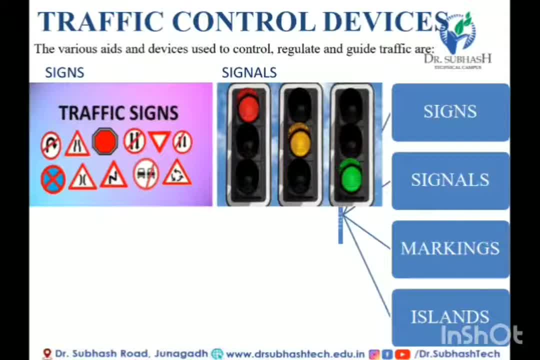 at important locations such as busy intersection, in order to regulate the flow of traffic, which includes everything from heavy commercial vehicle and cars to bicycle and pedestrians. however, these signals come with some rules associated with them. basically, the traffic signal rules form the very backbone of this science, and following them is vital for ensuring smooth and risk-free road travel. 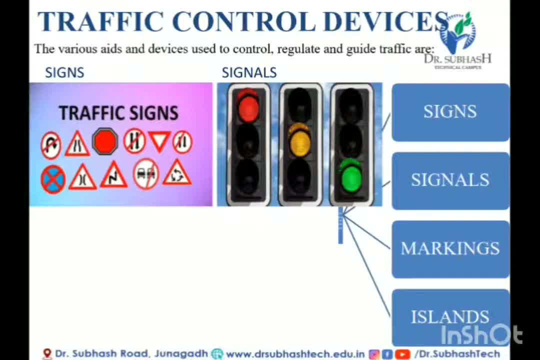 traffic signal is used as an instructing device that indicates the road user to act according to the displayed sign. now following. the traffic signal ensures road safety and to make things simple to understand this, traffic signals have been using a universal color code like red, yellow and green. red means to stop, yellow means the indication of the 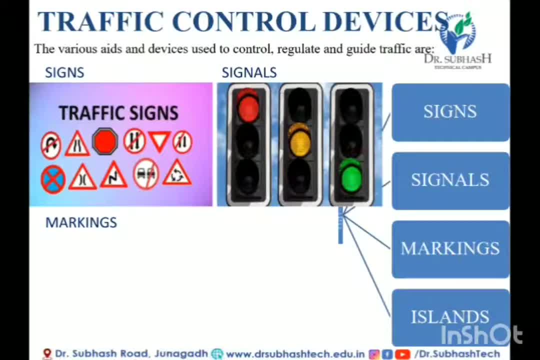 the red signal is about to be displayed and the green light indicates to go or to move forward. now the red light is generally the sign of danger or warning, and on traffic lights it signals a potential hazard ahead and hence is an indicator for the motorist to stop. also, you can turn left in a red signal only. 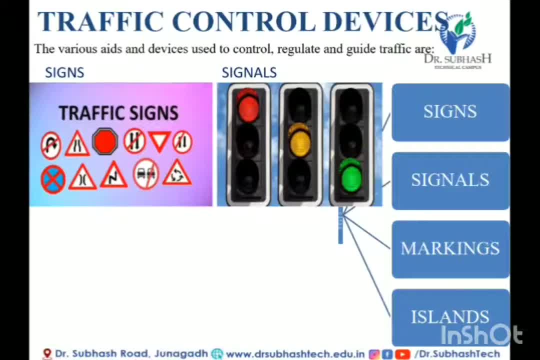 if there is a sign to do so. also, when doing so, you need to give the right way to pedestrian and vehicles that would be coming from opposite direction. a traffic signal that may aren't aware of is the red arrow, which basically means to stop until the green arrow appears, also a turn to the left, or in any other. 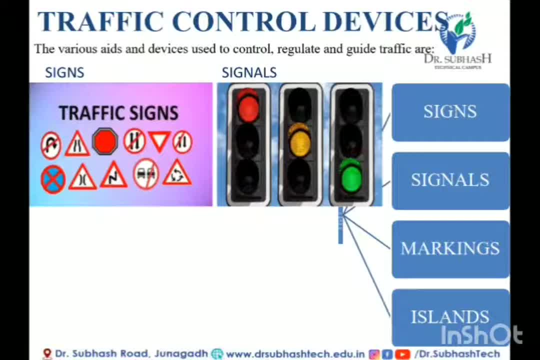 direction, for the red light is a sign of danger or warning that matter can't be made with. this signal is being displayed now. when there is flashing red light, it indicates the same as the stop light, which is basically top stop. once you have stopped, you can proceed ahead. after making sure 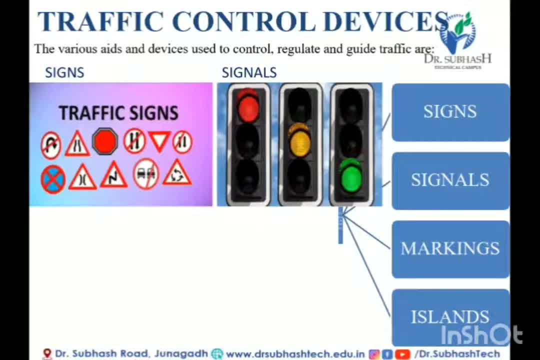 there is no obstacle in your path. now the yellow light, now the yellow traffic light, is a warning signal that lets you know that the red signal is about to be displayed. hence, when you see the yellow light, you should start slowing down to come to a stop, in anticipation of red light also, in case, for any reason, you can't stop. 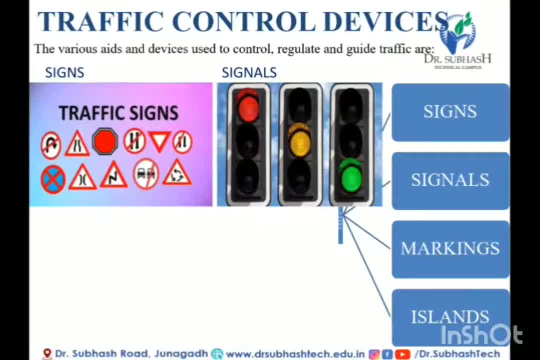 then you should look out for way girls that might be entering the intersection at the same time. so a yellow arrow indicates that the Red Arrow is about to be displayed, so one should stop on seeing this sign unless he is already in the intersection, and the flashing yellow light is basically a warning signal to. 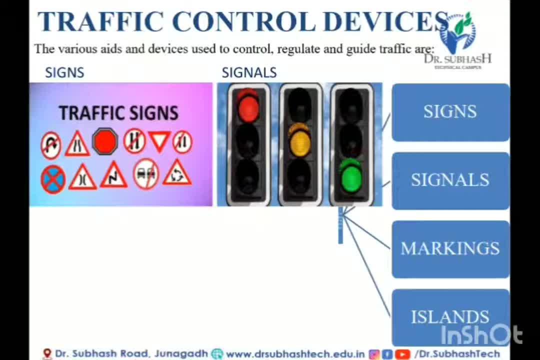 make the road users alert and slow down if needed. now talking about green signal, just like the red light corresponds to danger and stop, the green light signals safety and the word go. however, just to play it really safe, you should first let any vehicle remaining in the intersection pass before you go ahead. 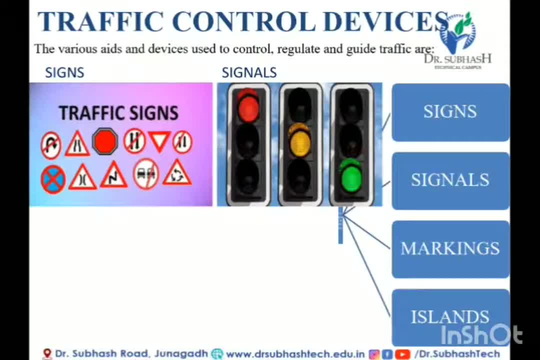 now, a green arrow means go, but first you must make sure that any vehicle, bicycle or pedestrian who is still in the intersection passes safely through it. also, a green arrow that points right or left will let you make a protected turn. there are six types of signal, that is, traffic control. 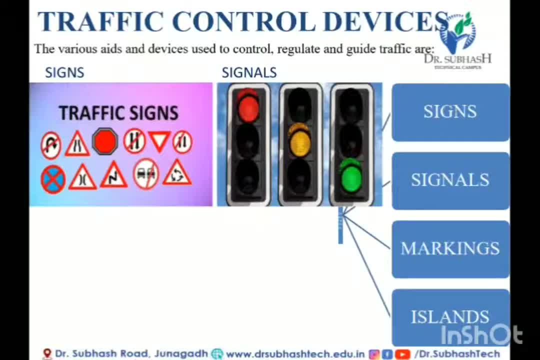 signal and traffic control signal and traffic control signal and traffic control signal, then fixed time signal, manually operated signals, traffic actuated signals or automatic signals, then pedestrian signals and special traffic signals. now the setup of traffic signal includes the controller, then traffic lights and detection. the controller works as the brain of the 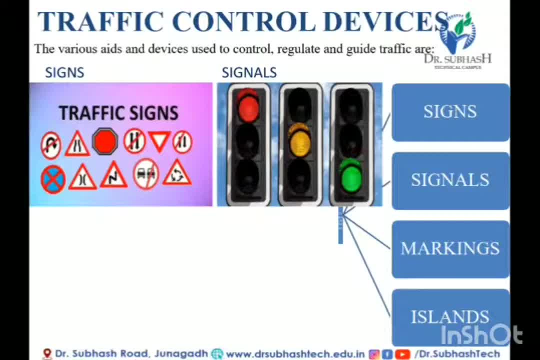 entire setup and has the information that is required to make sure that the lights work as per the required sequences. traffic signals can run under a variety of different modes, which can be dependent on the location and time of the day. now, apart from this traffic signal, the other kinds of signals are the: 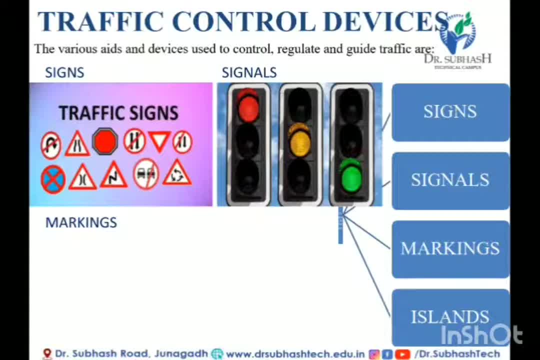 signals given by the traffic policeman in order to control the traffic congestion, and also the signals indicated in the vehicles, like if the vehicles want to turn left, then it will show a left inside indicator. so it is also important to know this kind of signals from vehicles as well as from the traffic. 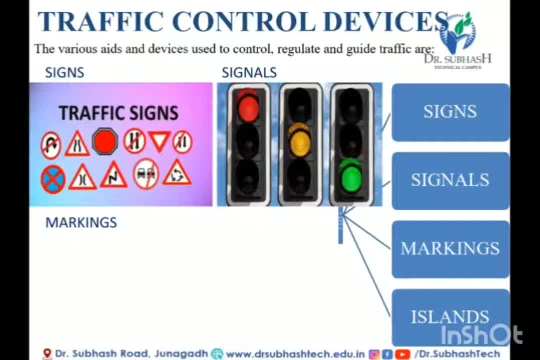 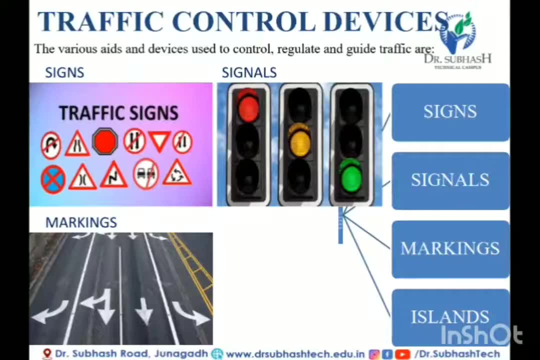 policeman. now the third type of traffic control device is markings, now road surface marking in� does not take much extra time and value. it means there is no title in terms of the marking is a kind of device or a material that is used on a road surface in order to convey. 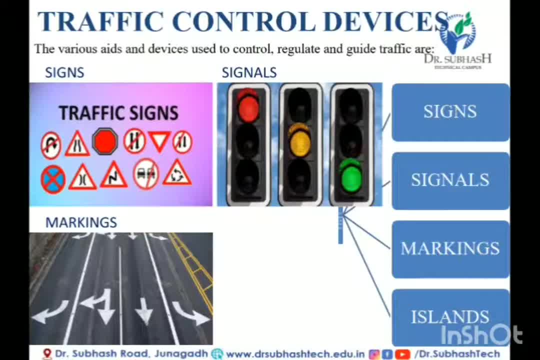 official information and they are commonly placed with the road marking machine or road marking equipment or pavement marking equipment. now they can also be applied in other facilities used by the vehicles to mark the parking space or designate the area for other uses. now road surface markings are used on paved roadways to provide guidance and information to the drivers. 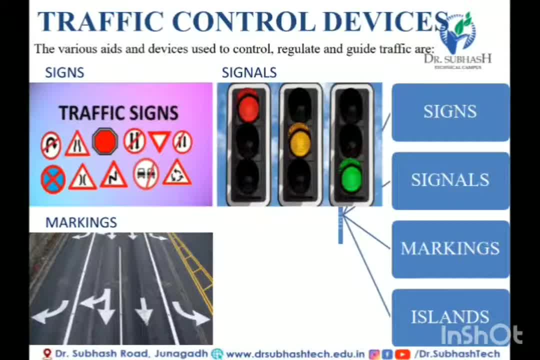 as well as to pedestrians. the uniformity of the marking is an important factor in minimizing confusion and uncertainty about their meaning, and efforts exist to standardize such marking across borders. however, countries and areas categorize and specify road surface marking in different ways. white lines are called white lines, mechanical, non-mechanical or temporary. they can be used to. 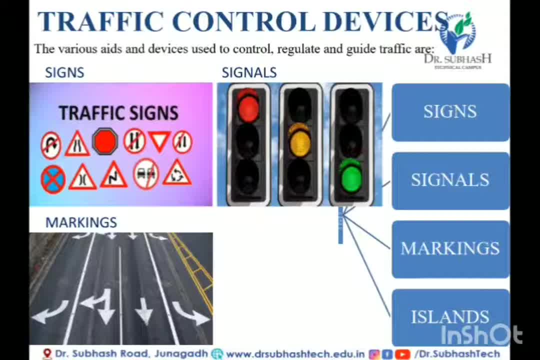 delineate traffic lanes, inform motorists and pedestrians or serve as a noise generator when run across a road, or attempt to wake a sleeping driver when installed in the shoulders of a road. road surface marking can also indicate regulations for parking and stopping. now there is a continuous effort to 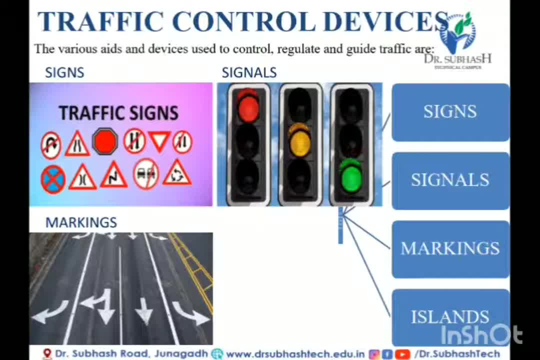 improve the road marking system, and technological breakthroughs include adding retro reflectivity, which increases the longevity and lowering the installation cost. today, the road markings are used to convey a range of information to the driver, spanning navigational, safety and enforcement issue, leading to their use in environment understanding, within the advanced driver assistance system and 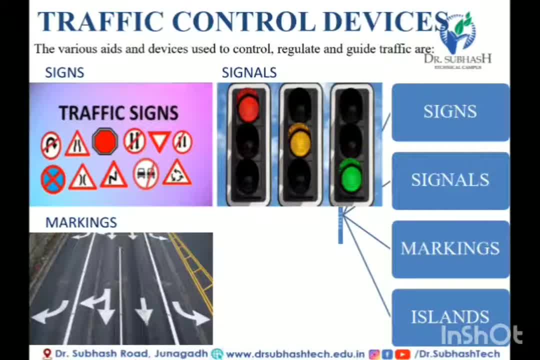 with state and federal immigrants driving participation for piloting vehicles to respond to месте problem scenarios. now let's talk about the information component. many of you may be familiar with the fao готов to inspired vehicle Road Warning and navigation system, one of the most important. 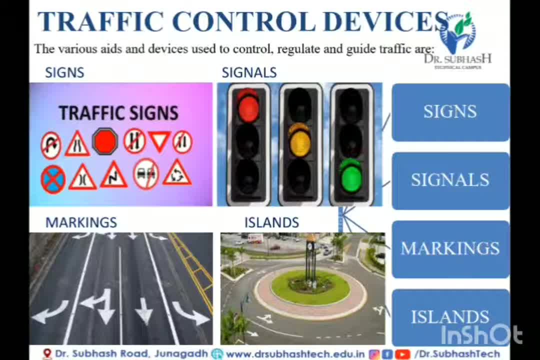 elements that is required for road traffic to be carried. Hoje there are various forms of road żeig direction around the central island and Bot init. after the road, ERA is encrones in hand the public parks in all the 8 Fresnoasiare. this makes full steps related to known volume. 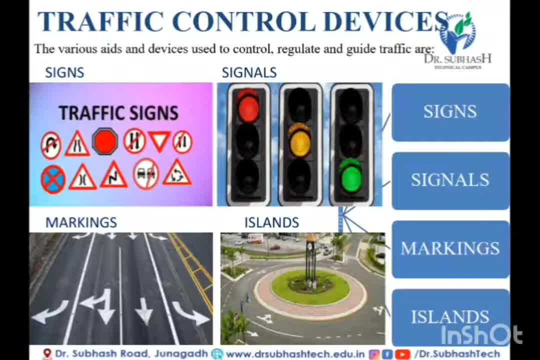 the traffic already in the junction. now modern traffic island observe various design rules to increase the safety. now, compared to stop sign, traffic signals and earlier forms of roundabouts, modern traffic island reduce the likelihood and severity of collisions greatly by reducing the traffic speed and minimizing the t-bone and the head-on collisions. variations on the basic concept include: 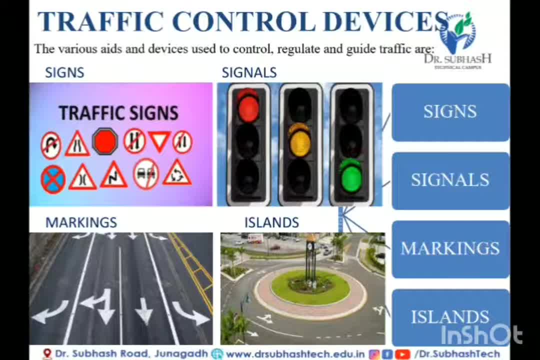 integration with tram or train lines to a flow, higher speeds and many others now traffic our traffic existing. the roundabout comes from one direction instead of three. simplifying the pedestrians. visual environment: traffic moves slowly enough to allow the visual engagement with the pedestrians. encouraging the difference to 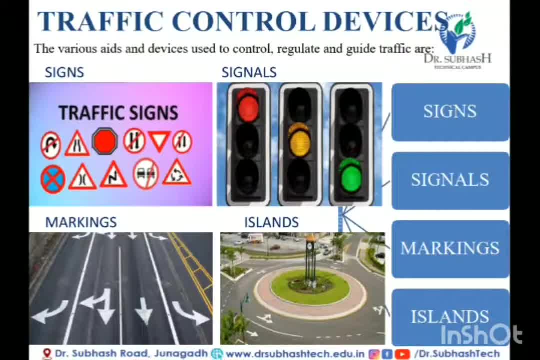 towards them. other benefits includes the reduced driver confusion associated with perpendicular junctions and reduced queuing associated with traffic lights. now, traffic island also allows u-turn within the normal flow of traffic, which often are not possible at other form of junctions. moreover, since vehicles that run on a gasoline averagely spend less time idling at traffic island than at 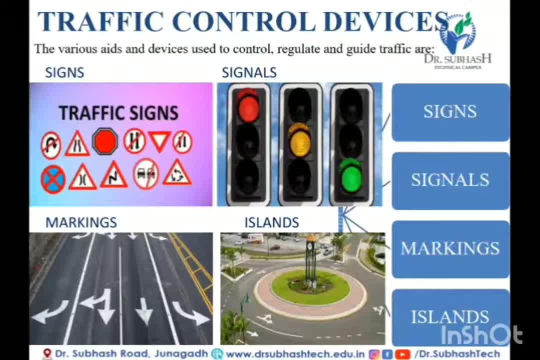 signaled intersections. using a traffic island potentially leads to less pollution. when entering, vehicles only need to give way. they do not always perform a full stop. as a result, by keeping a part of their momentum, the engine will produce less work to regain the initial speed, resulting in lower emissions. now, other than this, a traffic 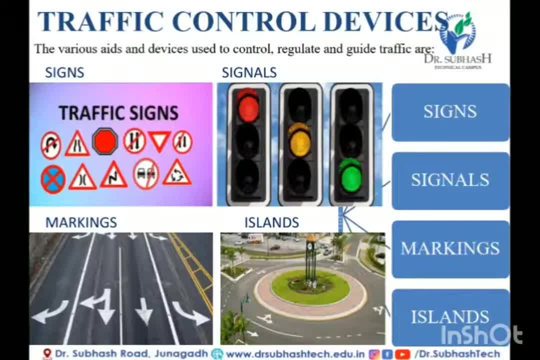 island is also a solid or a painted object in the traffic island, which is also a solid or a painted object in the traffic island, then it can also be a narrow strip of island between the road that intersects at an acute angle if the island uses the road markings only without waist curve or without other. 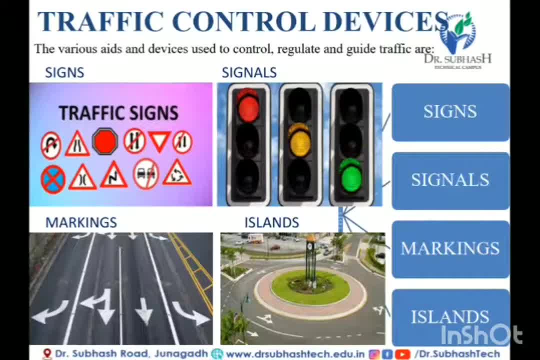 physical obstructions, then it is called a painted island or ghost island. Tasik Island can be used to reduce the speed of car driving through or to provide a central refuge to pedestrian crossing於 predestined crossing part of road, the road. now, when traffic islands are longer, they are instead called as a traffic medians. 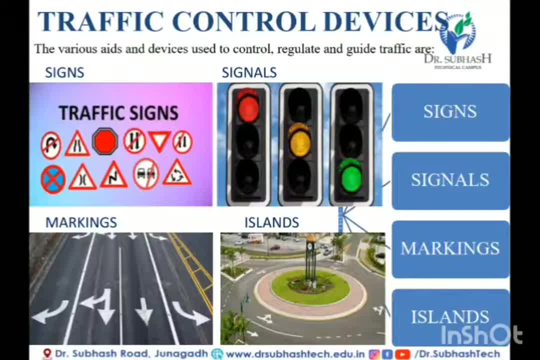 a strip in the middle of the road serving the divider function over a much longer distance. now some traffic island may serve as a refuge island for pedestrians. so these are the four main types of traffic control devices which are used to control the traffic. oh, now moving to the next slide. 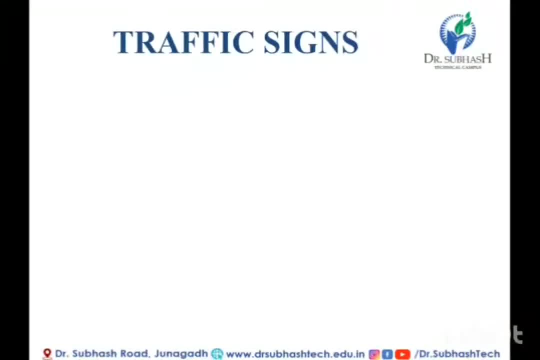 traffic signs. now let us study traffic sign in detail. so, traffic sign or a road sign are the signs erected at the side of a or above a road to give instructions or provide information to the road users. okay, so, as we have discussed in the previous slide the traffic signs, they are. 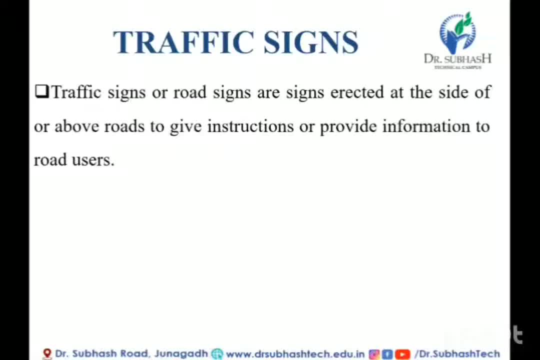 erected either at the side of the road or above the road, and the main purpose of providing or installing a traffic sign is to give instruction or provide information to the road users. informations like there is a one-way street or left turn is not allowed. certain kinds of 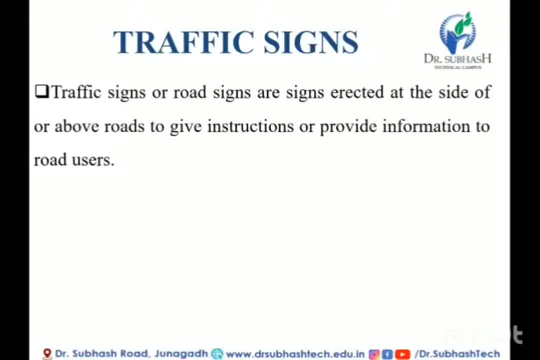 instructions and such informations are provided to the road users by installing the traffic signs. now, these traffic signs are used to ensure free movement of traffic and make the road users cognizant of specific laws and regulations, restrictions and prohibitions. so if all the road users will observe the traffic sign and follow them strictly, 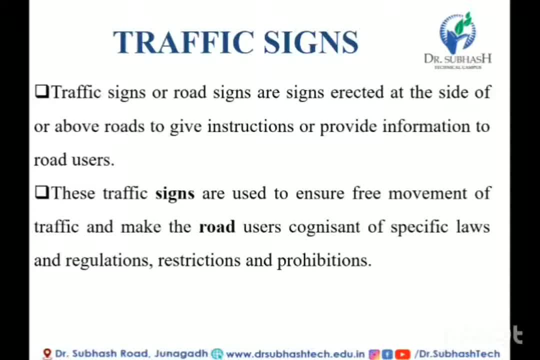 then it will ensure free movement of traffic with list conditions and list accidents, and it will make the road users to know about the specific laws, regulations, restrictions and prohibitions: prohibitions like no parking area, and specific laws and rules and regulations like speed limit. so these are the certain 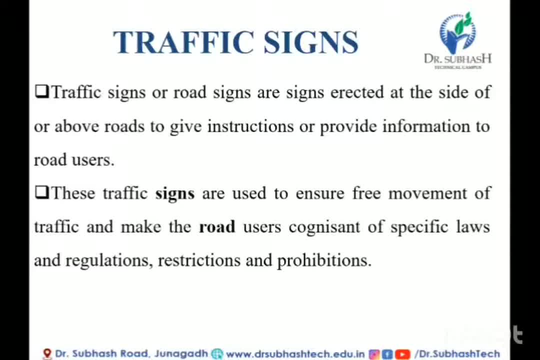 prohibitions or the information which the road users are given by providing or installing the traffic signs. now, neglecting the traffic sign, it can be dangerous and it may invite penalty. now, if you are not following the traffic sign, then you might meet with an accident or in case the traffic. 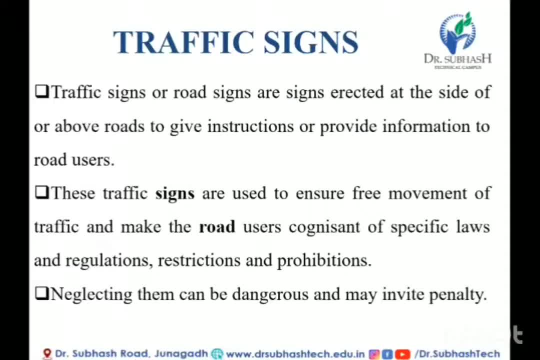 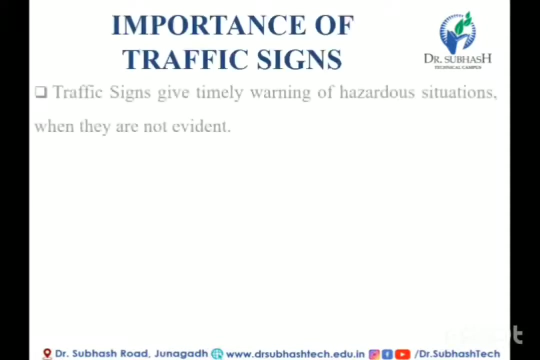 policeman observes that you are not observing the traffic sign, then they may charge penalty on you. so it is extremely important to follow the traffic signs in order to ensure safety and safety of the ensure smooth flow of journey. now moving to next slide: importance of traffic sign. 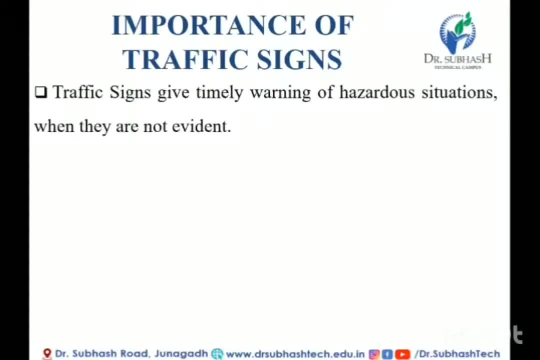 so traffic signs give timely warning of hazardous situations when they are not evident. now, a warning sign is a type of sign which indicates a stray traffic sign, like unusualру, a potential hazard, obstacle or condition requiring special attention. now some are traffic signs that indicate hazard on road that may not be readily apparent to 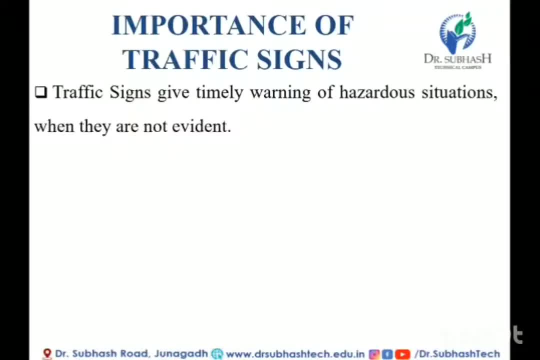 a driver. the warning signs usually contain a symbol. now many road signs warn you to slow down or watch for hazards or special conditions ahead. it might be a narrow bridge, it might be a sharp turn, it may be anything which is hazardous. so most of the warning signs are yellow and diamond shape with black. 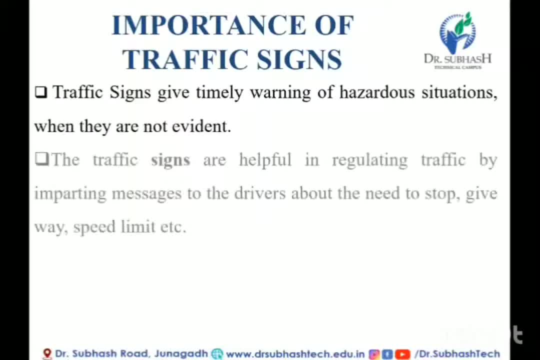 letters or symbol. now the traffic signs are helpful in regulating traffic by imparting message to the drivers about the need to stop, give way, speed limit, etc. now a stop sign is a traffic sign which is designed to notify the drivers that they must come to a complete stop and make sure the intersection is safely. 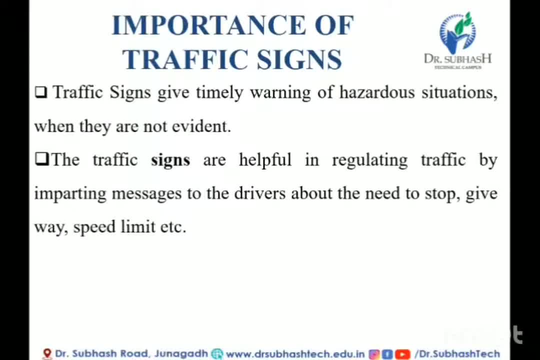 clear of vehicles and pedestrian before continuing past the sign. now talking about give way sign. now, when you come across a give way sign, then you must slow down and prepare to stop if necessary. a give way sign or a line means you must give way to all the vehicles traveling in, entering or 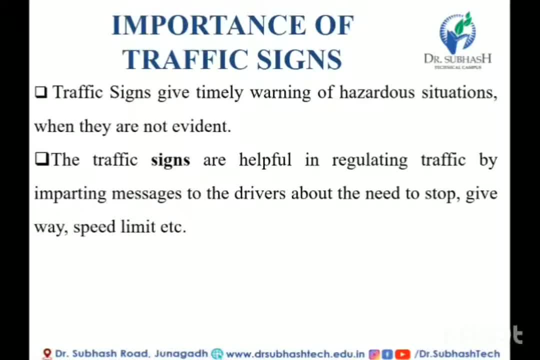 approaching the intersections, whether the vehicles are turning left or right or going straight ahead. now the shape of give way sign is upside down. triangle marking on the road represent a warning to the motorist that there is a give way just ahead now. speed limit sign is a regulatory sign now. 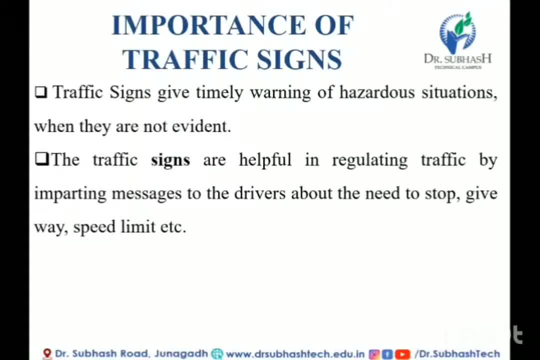 these signs are designed to communicate a set of legal maximum or minimum speed that the vehicles must travel. now, speed limits signs are generally indicated on a traffic sign reflecting the maximum or minimum permitted speed, and it is expressed as kilometer per hour or miles per hour. now the third importance of 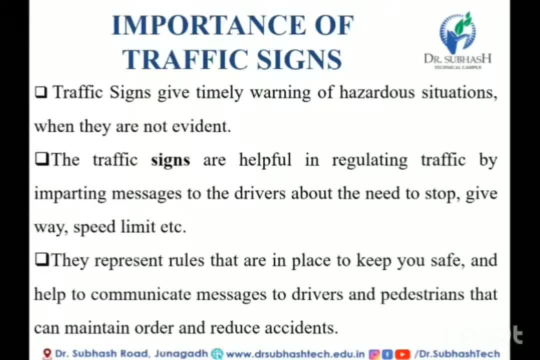 traffic sign is that they represent rules that are in place to keep you safe and help to communicate message to the drivers and pedestrians that can maintain order and reduce accidents. now, traffic accidents occur for various reasons, but the majority of traffic accidents are caused by the road users. 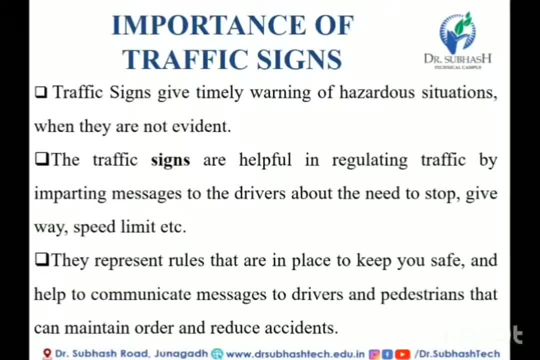 that is, by the drivers. drivers may fail to abide the regulations or if they don't consider the pedestrians and the other dangerous, hazardous situations, or if they don't follow the traffic signs which are installed, then it may invite accidents. so traffic signs is extremely important to keep you safe and